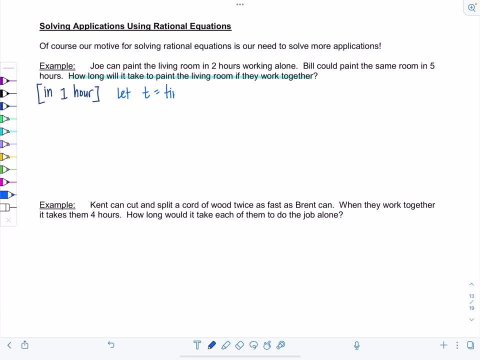 Equal how long or the time it takes to paint together. Okay, to get the whole job done. Okay. so what we want to do is figure out how much or what fraction of the job each of them is completing within one hour. So, Joe, it takes him two hours to paint the whole living room. 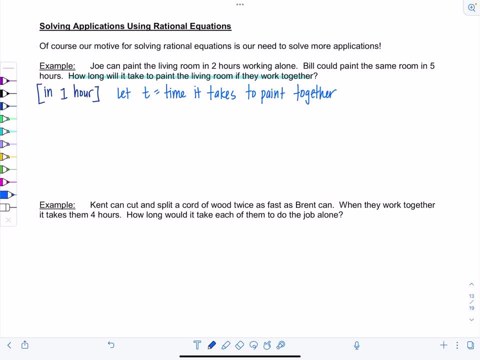 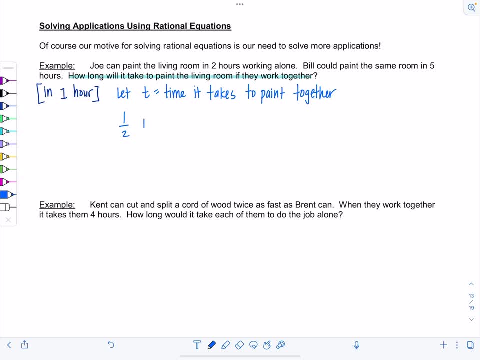 contribution. Okay, but Bill's also helping him. So I'm going to add to that the fraction that Bill gets done in one hour. So let's think Bill takes five hours to paint the living room. So after only one hour has gone by, how much has Bill finished? One fifth, So you basically do one over the. 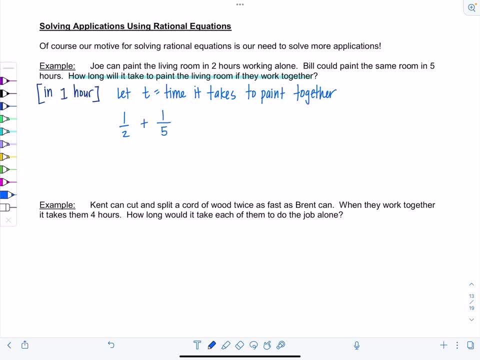 time right that it takes each of them to do the job by themselves, And so I'm going to set this equal to the fraction that gets done when they work together in one hour, which is one over t. I don't know how long it's going to take them to paint together, But one over t is going to be the. 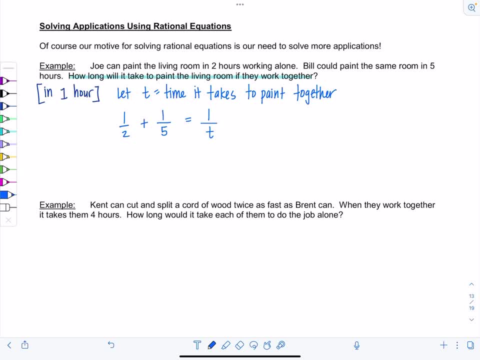 fraction that's completed by both of them, And this is our setup. That's it. So you'll notice this is a rational equation, like we solved in the previous video. So we're going to do one over t. So you want to list your restrictions? In this case, it's pretty obvious t can't be zero, But I 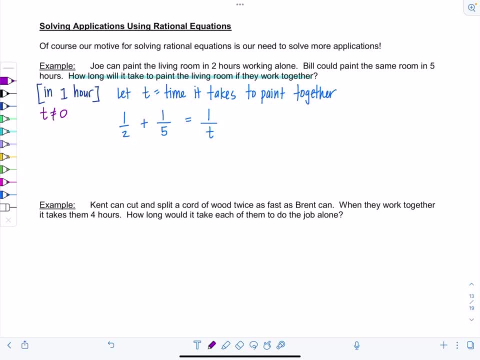 mean that wouldn't make sense as a solution. anyways, How could the job get done in zero hours? it just wouldn't get done. So usually the restrictions are kind of extreme and not too worrisome for a lot of these. Next up we're going to multiply by the LCD. So two, five and t gives 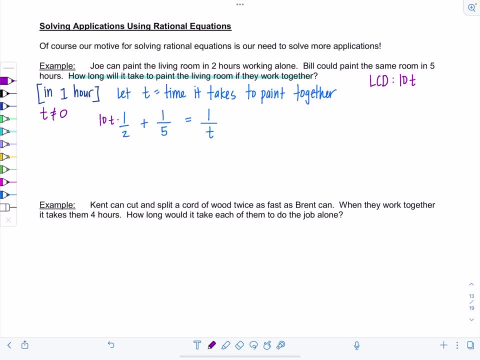 us 10t. I'm going to multiply everything in the equation by 10t in the numerator. Remember: if you need to add an over one, go for it. I usually don't so it doesn't get messy, But if you need it as a reminder, be my guest. Okay, so the two is going to cancel with the 10.. 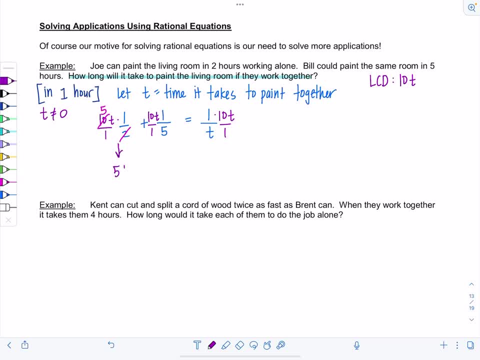 We've got 5t over here Plus let's see what else cancels Five and 10 cancels, So then that's just 10t equals on the right hand side the t cancels, So I just have 10.. Oh, what a harmless little. 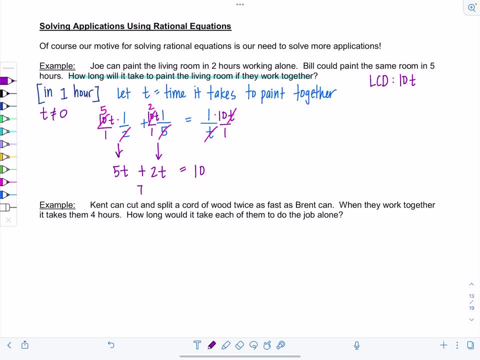 equation we have here. Love it. So this gives us: 7t equals 10.. So t equals 10. sevenths hours, right? Make sure you put units. So just ask yourself: does this make sense? Joe takes two hours by himself And this is less than two hours. 14 over 7 would be two hours, So 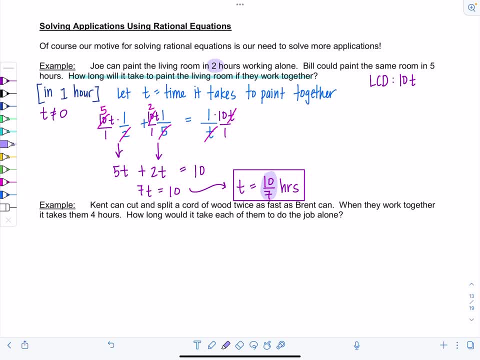 this is less, which makes sense because Bill's helping you. It shouldn't be more than two hours, unless Bill's doing something wild like you know, throwing paint all over the walls and on the carpet and causing a mess, But didn't say anything about that. So, yeah, looks like everything's. 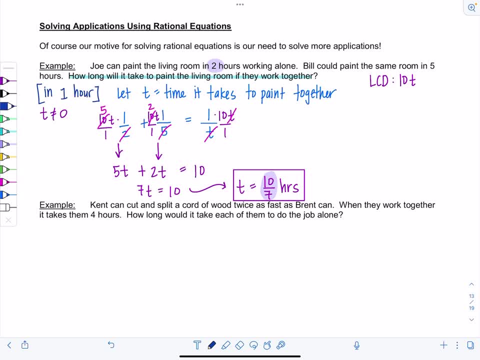 checking out. Some instructors want you to write a sentence for your final answer, Whatever. So if they do, then you could just say it takes 10 sevenths hours together, or whatever. Okay, Good, Let's just highlight that and move on. 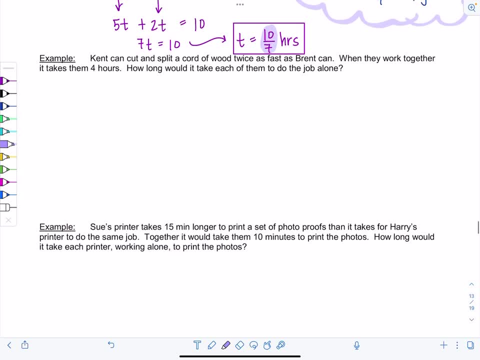 Another similar work setup. Okay, Kent can cut and split a cord of wood twice as fast as Brent can. When they work together- together, it takes them four hours. how long would it take each of them to do the job alone? okay, the word twice as fast can be confusing because you have to think who's slower. 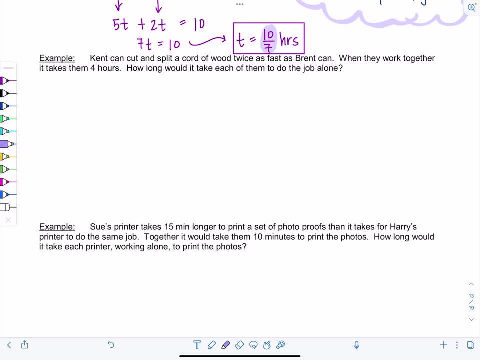 kent can cut and split a cord of wood twice as fast as brent can, so that means brent is slower. brent is slower, so let's let x equal the time it takes for kent, and since he's twice as fast, that really means he does it in half the time. so brent takes two x. 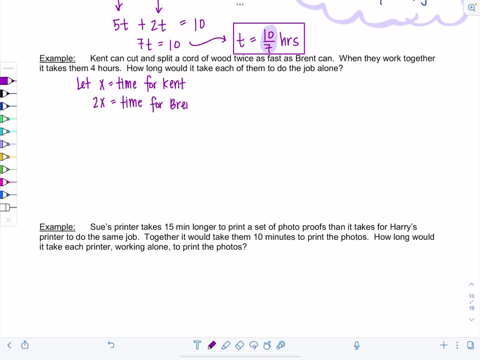 okay, slow poke brent. okay, how long would it take for each of them to do the job alone together? we know that it takes them four hours. how long would it take for each of them to do the job alone? them four hours. so a little bit of a different setup than last time, but same idea in one hour. 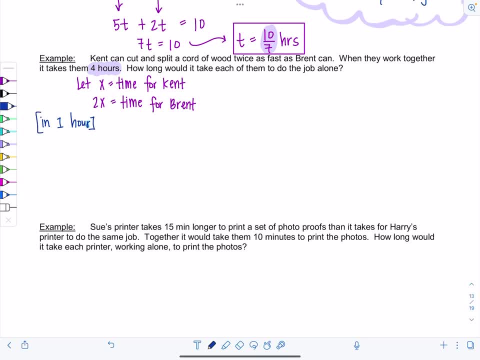 in one hour you guys tell me what fraction of the job has kent completed after one hour? it takes him x hours, so one over x, plus brent is helping, so one over two x is contributed by brent. thank you, brent, and this is gonna. 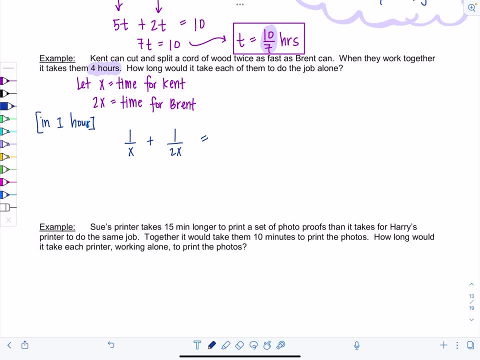 equal the fraction that they get completed together in one hour. well, it takes them four hours together to get the whole job done. so after one hour, one-fourth of the job is done. all right, good. so now we've got our equation. that's usually the hardest part for students. 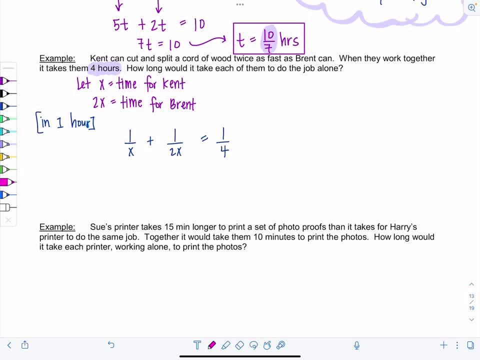 is just setting up the equation and let's list our restrictions: x can't be zero and then multiply through by the lcd. so lcd is just going to be 4x, right? 4x, 4x, 4x. so we're gonna be left with 4x times 1 over x. x cancels this is just 4, 4x over 2x. i'm gonna have a 2 left over equals x. 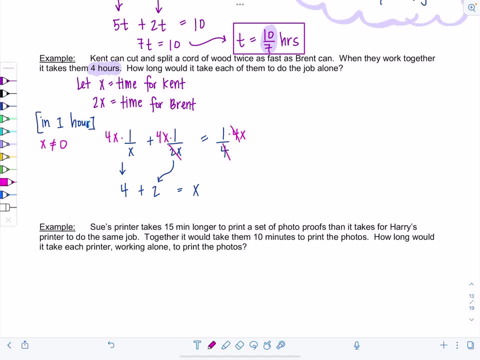 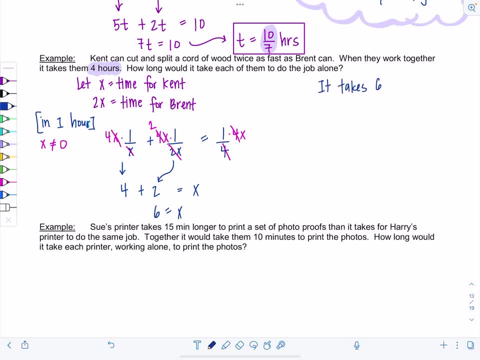 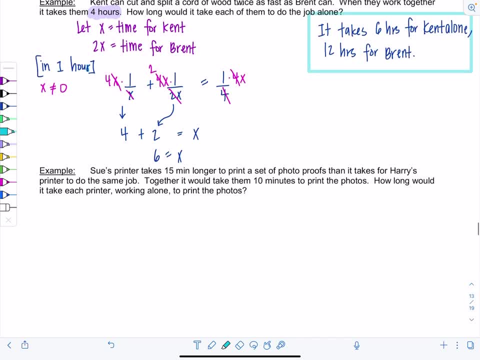 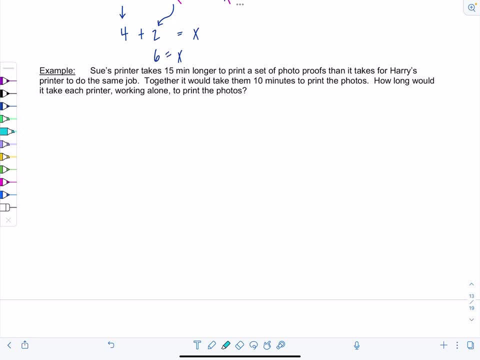 all right, i got one more work problem for you. once you do a few of these you realize they're all basically the same and they're not so scary. soos printer takes 15 minutes longer to print a set of photo proofs than it takes for Harry's printer to do the same. 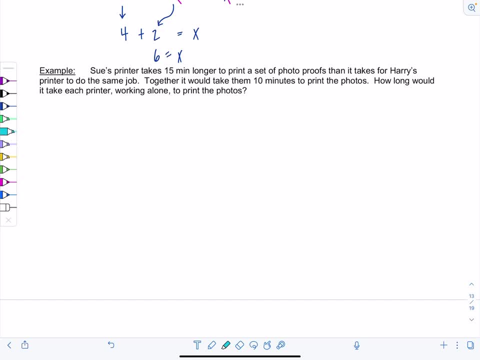 job Together. it would take them 10 minutes to print the photos. How long would it take each printer working alone to print the photos? So we don't know how long it takes Sue's printer or Harry's printer- And a good piece of advice when you're trying to figure out which one should I. 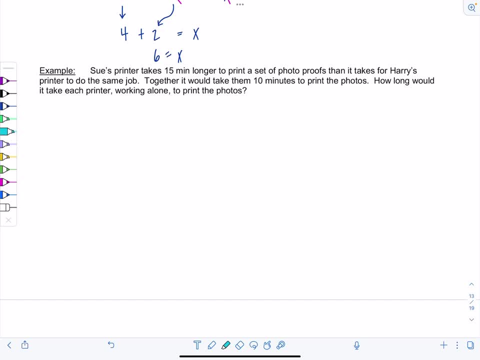 let x equal. let it be the one that you have less information about from the word problem. So what do I mean by that? See how they're telling you all this stuff about Sue's printer. Oh, Sue's printer takes 15 minutes longer. Okay, I don't know anything about Harry's poor little. 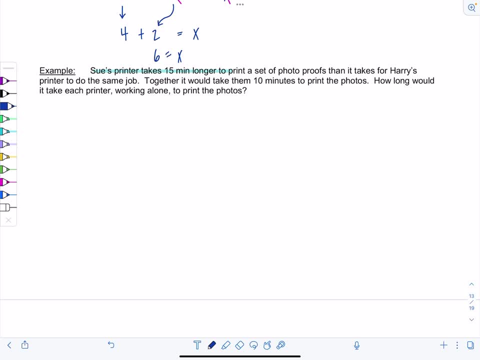 printer. So that means it's going to be easier if I let x equal the time it takes for Harry's printer. Okay, and then naturally you can see: okay, Sue's printer takes 15 minutes longer, So that means x plus 15 is going to be the time. 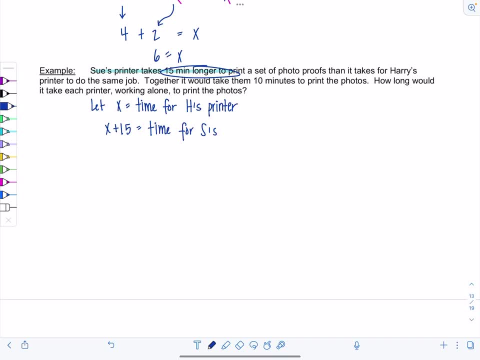 It takes for Sue's printer working alone. Okay, so when deciding what quantity x should equal, usually pick the. you know the quantity or the person or the amount that you have less information about. Okay, so this time the problem is working in minutes, not a big deal. 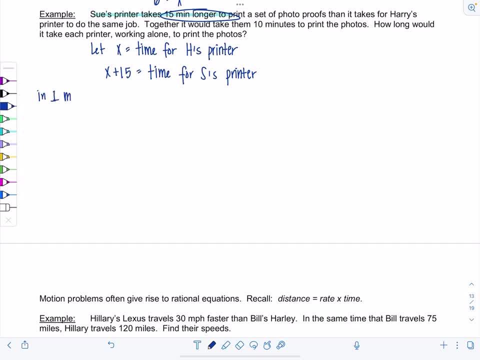 So in one minute we want to look at how much of the job, the printing job- gets completed One minute. Okay. so in one minute Harry's printer has completed what fraction of the job? One over x, Good. And what about Sue's printer? One over x plus 15. Excellent. 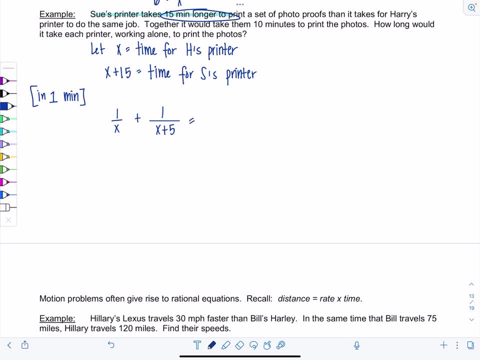 And this is equal to: did you catch how long it takes for the two of them together? Ten minutes, Okay, so this is going to equal one-tenth. Now let's list our restrictions: X cannot be 0 or negative 5.. 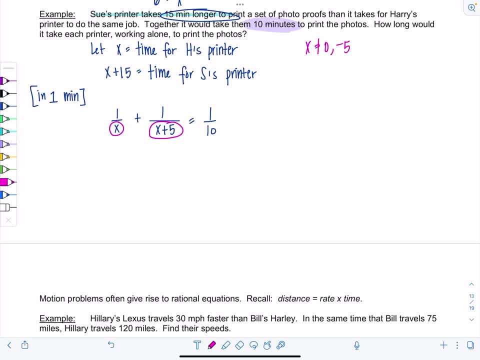 I mean x is time, so it wouldn't make sense for it to be 0 or negative. Oh 15.. Why do I have a 5 down there? Excuse me, Were you all screaming at your computer screens right now? 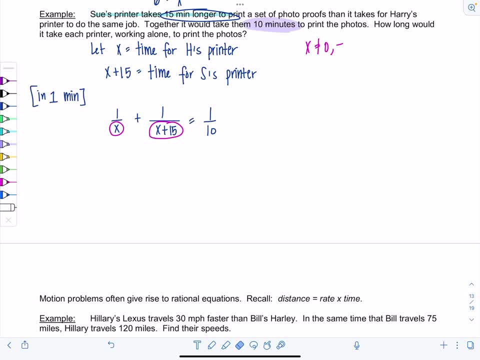 X cannot be negative 15.. Okay, it wouldn't make sense for it to be negative, right? Okay, good, Now let's multiply everything by the LCD, Which, in this case, is going to be all three denominators multiplied by each other, right? 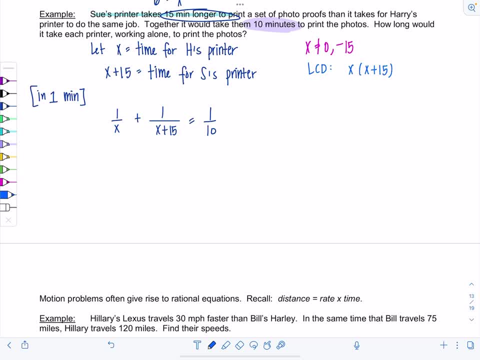 x, x plus 15.. Let's put the 10 in the front so it looks nice. So 10x times x plus 15.. And then here too, 10xx plus 15 and 10xx plus 15.. Okay, First term over here. what cancels? Just the x, right. So you have 10 times x plus 15. 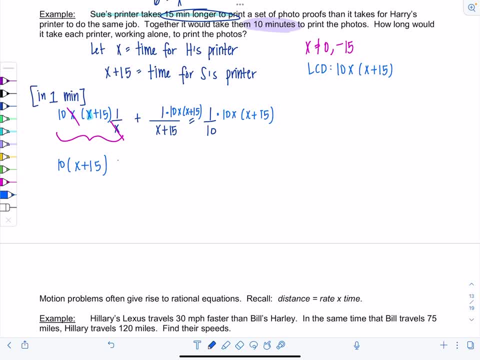 plus what cancels over here on the next term. x plus 15 cancels. so I have 10x And then this equals: cancel the 10,. I just have x times x plus 15.. Okay, Make sure at this step you don't have any more denominators, right? Otherwise you messed. 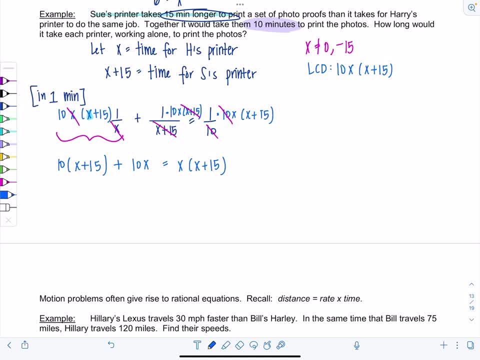 up somewhere. like you didn't multiply by the LCD correctly, you didn't pick the right LCD, something went wrong. The goal is to be fraction free at this point. Let's just distribute now. So we've got 10x plus 150 plus. 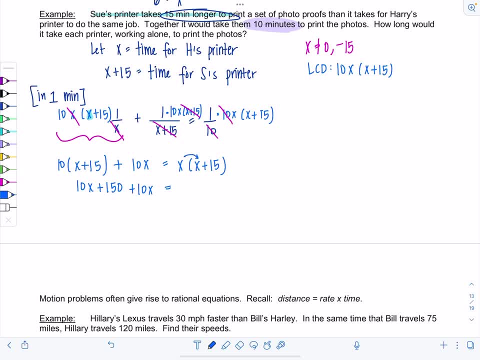 10x equals. if I distribute this x, we're going to have x squared plus 15x. Guys, as soon as you see you've got an x squared, it's time to set the equation equal to zero. So we've got 20x on the left-hand side. If I move them over to the right, 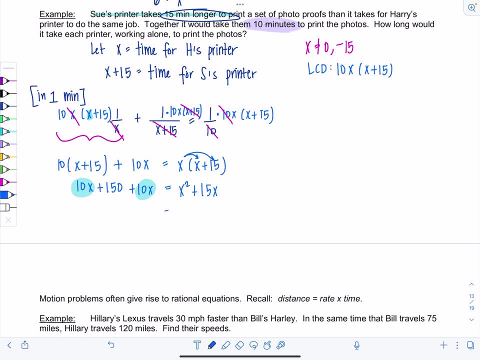 then I'm going to subtract 20x, So we've got x squared: 15 minus 20 is going to be negative 5x and then minus 150.. You know why I moved everything to the right? Because I wanted to keep that x squared positive. Oh yeah, that way I can easily factor now. So can you think? 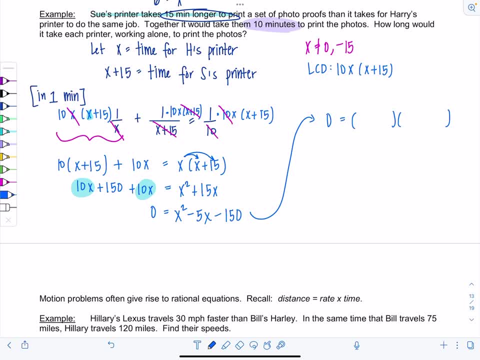 of two numbers that multiply to 150, negative 150, and add up to negative 5? Yeah, 10 and negative 15.. So x plus 10, x minus 15.. Good, So, setting each factor equal to zero, you get either x is negative 10 or x is 15.. 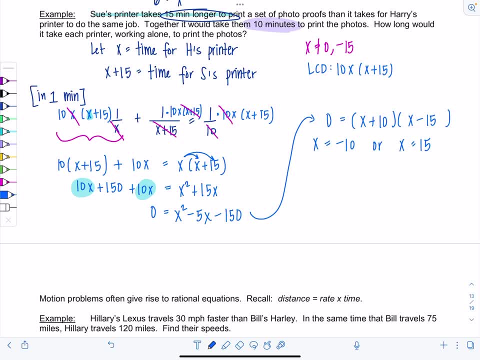 Both of them will not work. And think about it: x is time. We can't go back in time yet, So it doesn't make sense for x to be negative 10.. Okay, so our only solution is: x equals 15.. 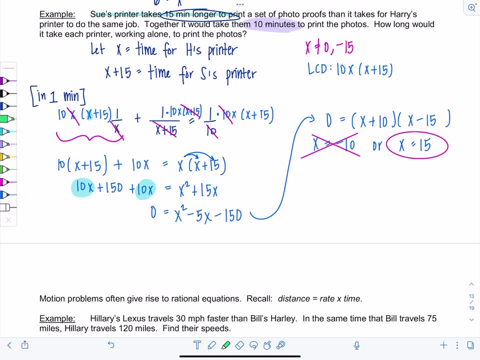 And then let's make sure we answer the question like obedient little math angels: How long would it take each printer working alone to print the photos? Okay, so Harry's printer would take 15 minutes And Sue's would take 15 plus 15, right? 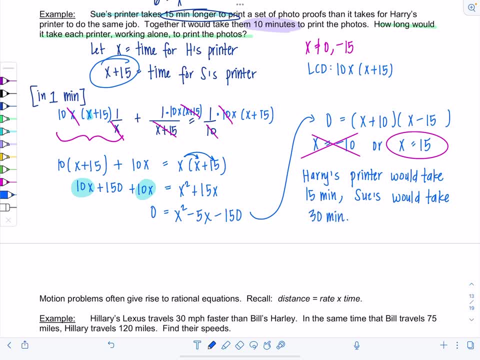 Okay, 30.. 30 minutes, My goodness. Okay, Very good. So these are just some examples of work problems. There's plenty more, But the more of these applications, word problems, whatever you do, you start seeing patterns And then you'll recognize how to set them up and that they're 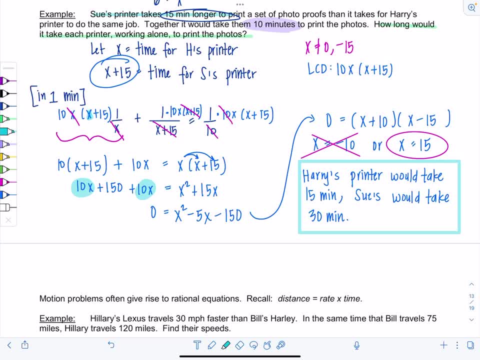 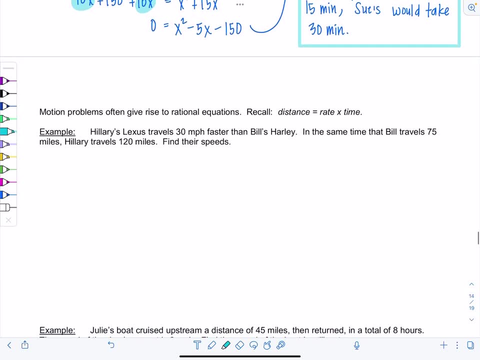 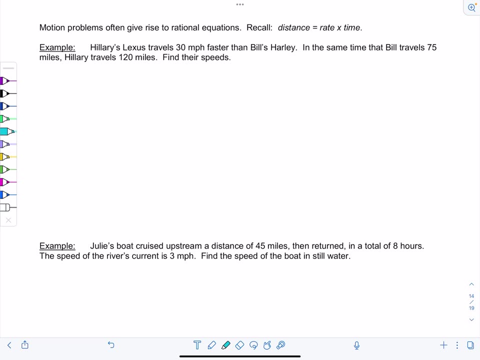 all essentially the same problem, Just, you know, put in different scenarios. Okay, another technique: This type of rational equation that comes from a word problem has to do with motion and using distance equals rate times, time. For these ones I do like to make a table. I think it helps organize. 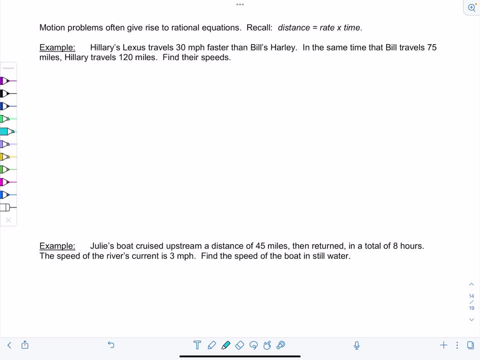 all the information. So, first example: Hillary's Lexus travels 30 miles per hour faster than Bill's Harley. Go, Hillary. In the same time that Bill travels 75 miles, Hillary travels 120 miles per hour. Find their speeds. So we need Hillary's speed and Bill's speed. Okay, what I'm gonna do is make a table. 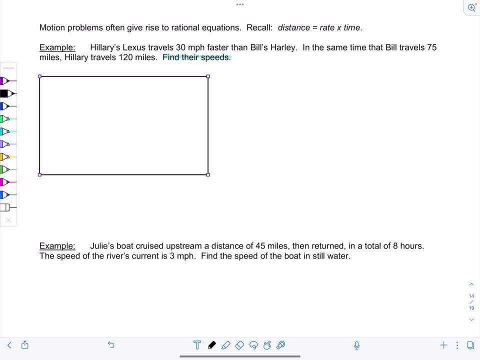 just to help organize everything and set it up this way, We've got two rows, one for Hillary and then one for Bill, And you're gonna have distance equals rate times time. So three columns in the table, two rows, One for Bill, Two rows, two rows. Three columns in the table, Three rows, two rows. 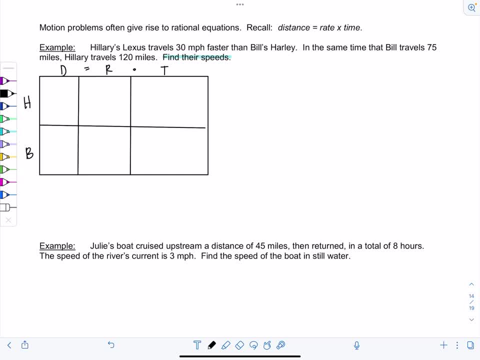 one for Hillary, one for Bill, And we're trying to find each of their speeds, okay, Each of their rates, basically. So one of them is going to be X. You got to go. oh, is it Hillary's speed? that? 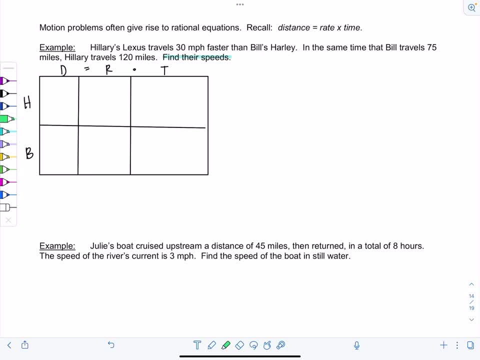 should be X, or is it Bill's speed? So let's read the problem again, see who they gave us less info on. They told me all this stuff about Hillary and her Lexus. It's going 30 miles per hour faster than Bill's Harley, but I have no info on Bill's Harley, So let's let X equal the speed of Bill's. 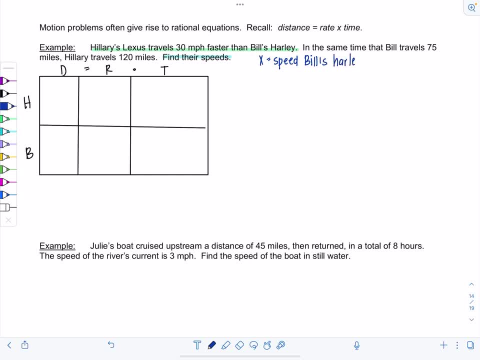 Harley. okay, And then what would Hillary's speed be? Her Lexus goes 30 miles per hour faster. Good, X plus 30 would be the speed of Hillary's Lexus. Okay, so I'm going to fill that in for the rate column for each of them. 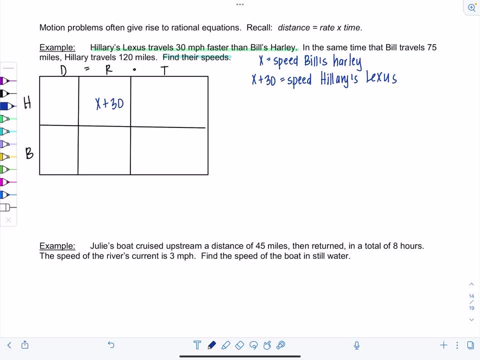 So for Hillary we're going to put in X plus 30, and for Bill just X. Okay, and then the problem says in the same time that Bill travels 75 miles. okay, so Bill distance 75,, Hillary travels 120 by their speed. Well, what the heck The time. 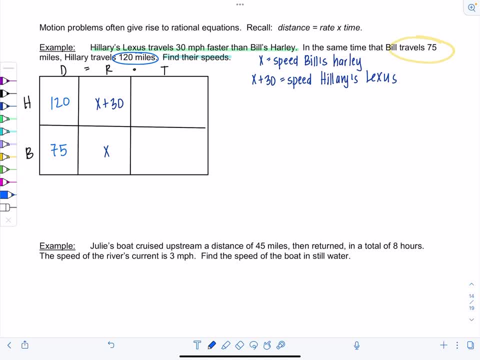 column is missing. That happens, Don't freak out. This is where you go back to the fact that we know distance equals rate, times, time. So if you rearrange and try to get time by itself, you would divide both sides by R, Yeah. 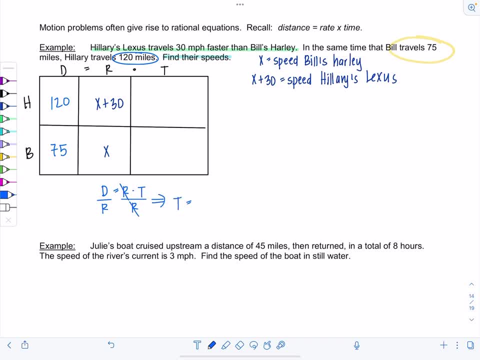 cancel, cancel. So that means time equals distance divided by rate. So for the time for Hillary, you're going to take her distance 120, and divide it by her rate X plus 30. And then similarly for Bill: for his time, you're going to put his distance 75, divided by his rate, which is X. 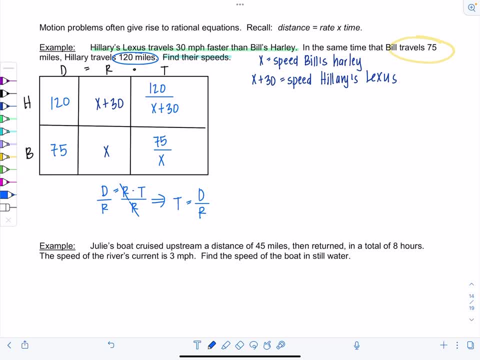 Okay, good. So we've got this cute little table filled in, but it does us no good until we can write an equation with it. right? There's still one more piece of info we haven't used from the directions. Did you catch it? You have to be a little detective, It says. 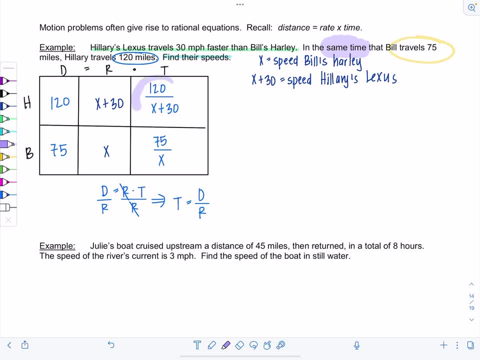 in the same time. So that means Hillary's time is the same or is equal to Bill's time. Okay, So that's the basis for which we're going to build our equation. We're going to set 120 over X plus 30, equal to 75 over X. It's not always going to 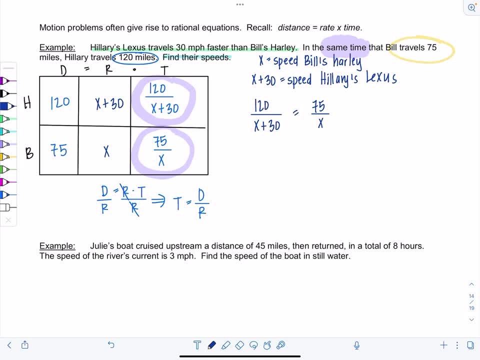 be the case that you're going to set the times equal to each other, That you know how to write. the equation is specific on each individual word problem, but there will be information in there to help you out. So that's the basis for which we're going to build our equation. 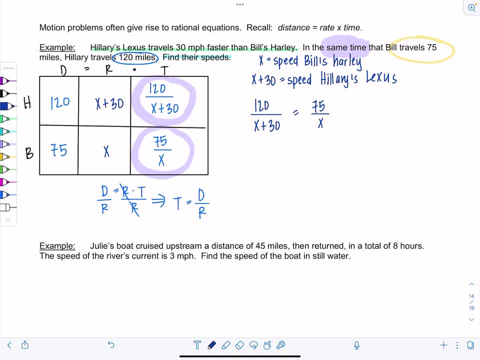 help you figure out what equation to write what's appropriate, okay? So here we've got a rational equation. I'm going to list restrictions, even though they're kind of obvious, like x can't be 0 or negative 30. I don't think any of them would be at a standstill or traveling backwards. 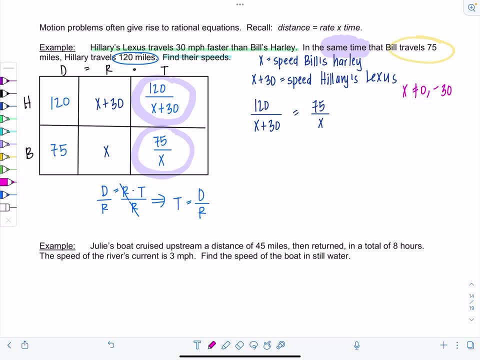 okay, But here we go. You can clear out the fractions by multiplying by the LCD. or you see how we have just one rational expression on one side and then one on the other side. You can take a little shortcut and cross multiply So you can do: 120 times x equals 75 times x plus 30.. 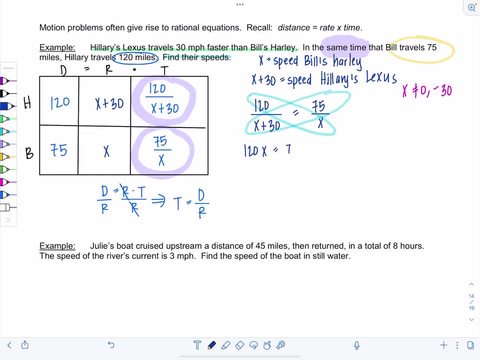 Oh, how fun. So 120x equals 75 times x plus 30.. And then, like what a non-frightening equation this has become right. Distribute So 120x equals 75x plus 75 times 30,, 2,250.. Okay, what to do next to solve you guys? 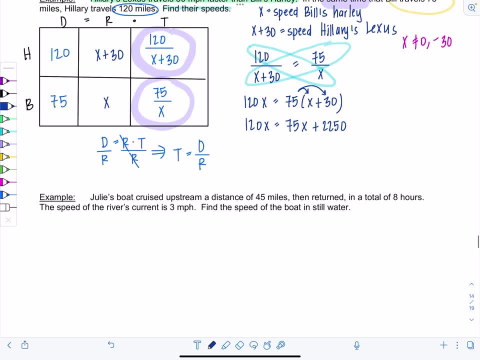 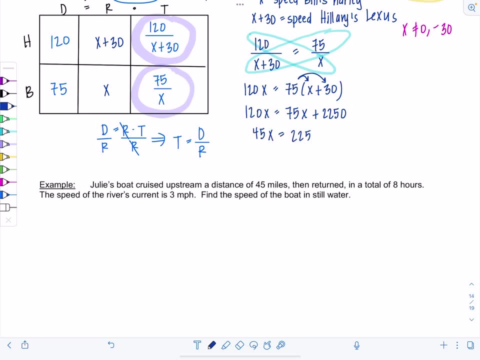 Good, Put all the x's on one side. So I'm going to subtract 75x. So we have 120 minus 75, that's 45x equals 2,250.. Divide by 45, x is equal to 50.. 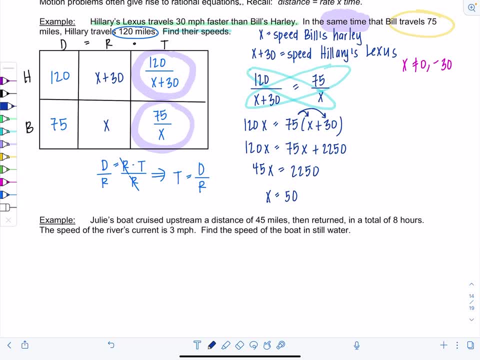 Okay, so let's answer the question. Find each of their speeds. So Bill travels at 50 miles per hour And Hillary travels at x plus 30, right, Remember that was her rate. So 50 plus 30, that's going to be at 80 miles per hour. 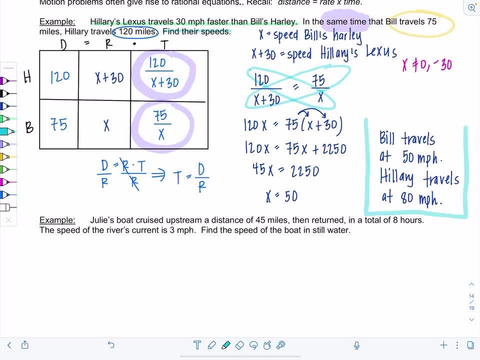 Which, frankly, in California, that's how fast everyone drives on the freeway. Okay, Good, One more rate problem where we're going to make a table. Okay, are you ready? It comes up quite often, this little scenario, So here we go. Julie's boat cruised upstream. 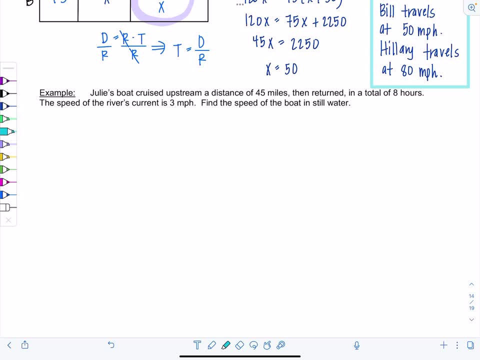 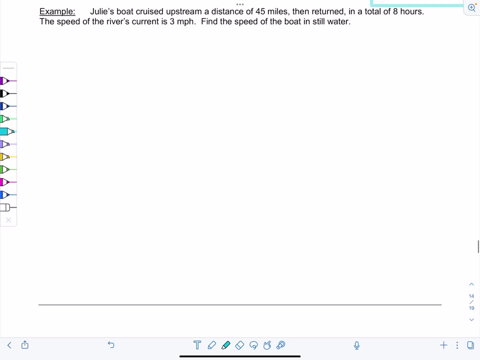 a distance of 45 miles. Look at Julie cruising And then returned in a total of eight hours. The speed of the river's current is three miles per hour. Find the speed of the boat in still water. So we're going to make a table here. We're going to have again two rows, one for when Julie is. 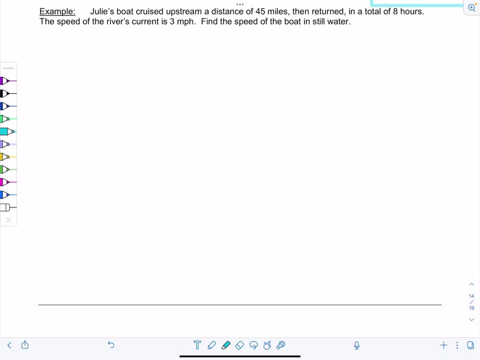 cruising upstream, and then one for when she's cruising downstream And we're going to use again, distance equals rate, times, time, And then let's see if you guys can figure out what the variable should be. Okay, so here's my cute little table. 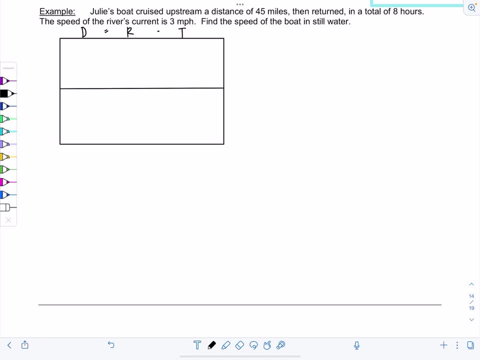 Distance equals rate times time. One is for upstream, One row, and then one row is for downstream. Okay, notice, we're asked to find the speed of the boat in still water, So there's a current in the river. they want to know how fast the boat just traveled on it's. 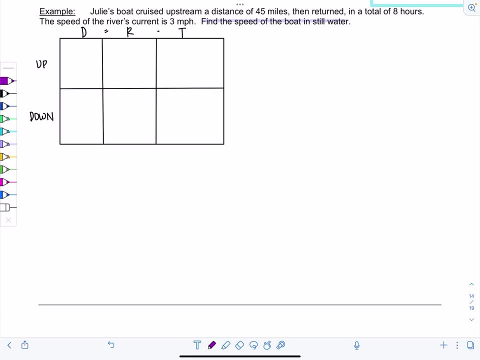 own if there was no current, if there was still water. So there's only a 10 minute delay water. So we're going to let x equal the speed of the boat in still water. Okay, good, So let's see. 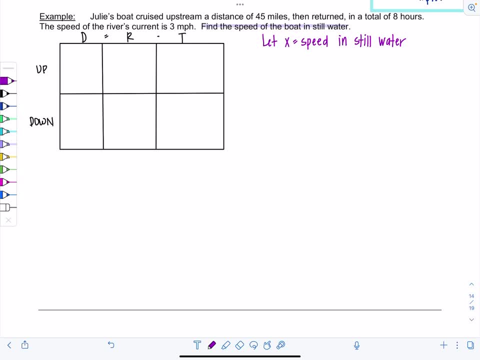 here. She's cruising upstream a distance of 45 miles and then returns, So the distance upstream and downstream is going to be the same. She's going 45 miles each way. Okay, what about the rate? The speed of the river's current is three miles per hour, So the rate here is going to be. 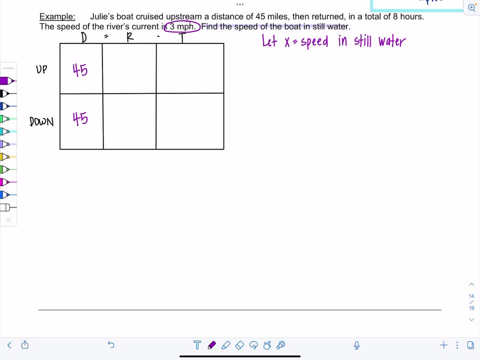 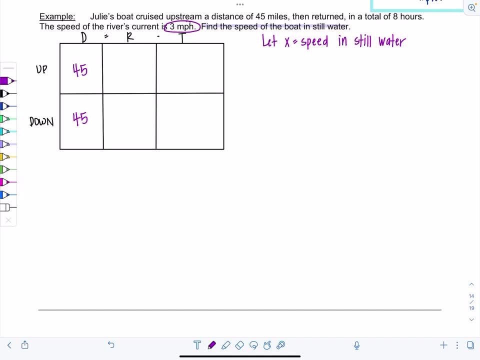 That means her net speed or her rate is going to be x minus three. You have to have minus three second. You can't write three minus x because that would mean that you're going backwards. basically, It always has to be the greater quantity first. So if she's getting anywhere, that means her boat. 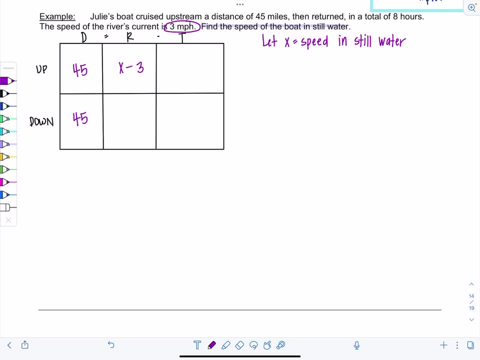 goes faster than the current And then downstream. now the current is helping her, So the rate is going to be x plus three. They're working together, speeding her up, And then time we don't have. You don't bust out another variable. Who wants that? Keep it simple. One variable makes. 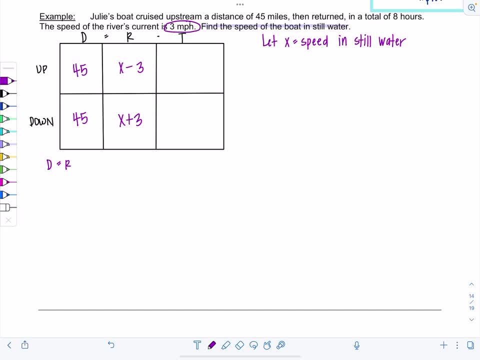 us happy. So again, since we know distance equals rate times time, we can use the fact that time equals distance divided by rate. So time upstream is going to be 45 over x minus three, And then time downstream, 45 over x plus three. Very good, Okay, do we set them equal to each? 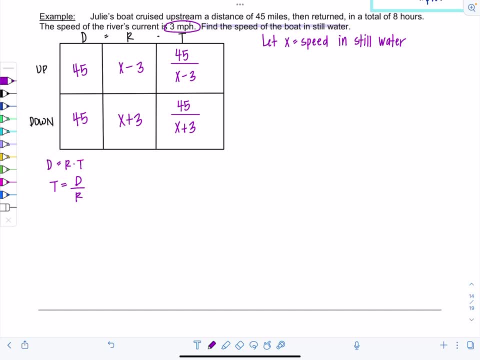 other, like the last problem That sounded so fun. No, no, no, no. It says the trip upstream and downstream took a total of eight hours. Hmm, So that means this time plus this time equals eight hours. Good, So writing the equation will be different. every word problem. The setup for the table, though. 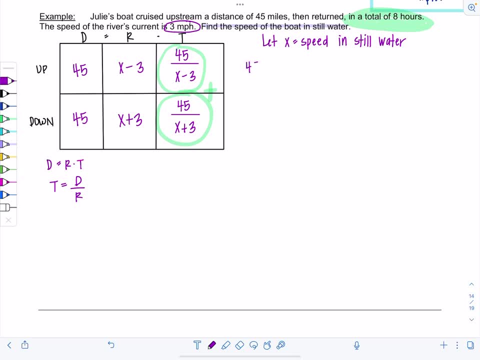 is pretty much uniform. So now we've got 45 over x minus three plus 45 over x plus three equals eight. Okay, we have restrictions: X can't be plus or minus three, but that makes sense. Can't be negative three. 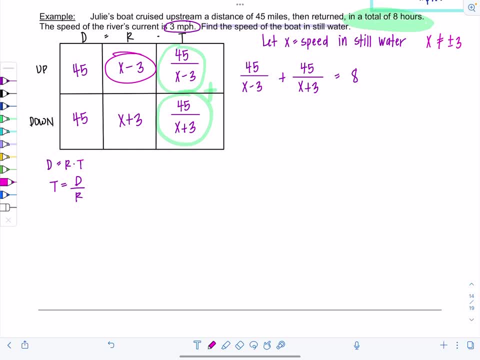 If she only went three miles per hour, that means it would be going nowhere when she's going upstream, which makes no sense. Okay, let's multiply by the LCD. Did you figure out what it was? This eight is over one, So we're going to multiply everything by x plus three. x minus three. 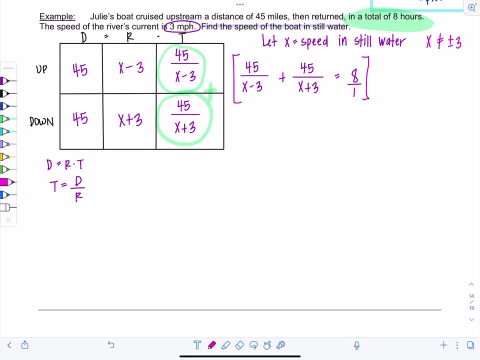 You guys, I'm going to show you what I do with the more advanced students. You can just put brackets around the equation, put the LCD out here once and then in your mind you're going to distribute and cancel. Okay, you can handle it. Watch this. So x minus three. 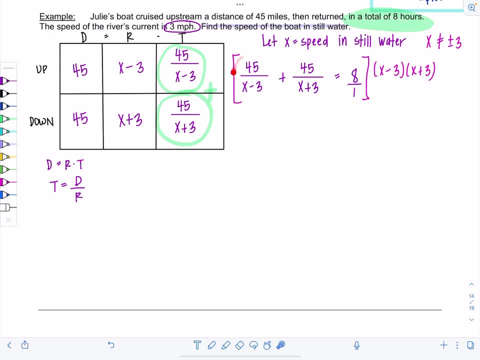 times x plus three. If I multiply by this first term, 45 over x minus three, the x minus three will cancel out. So all I have left is 45 times x plus three, Plus We okay Good Next term. 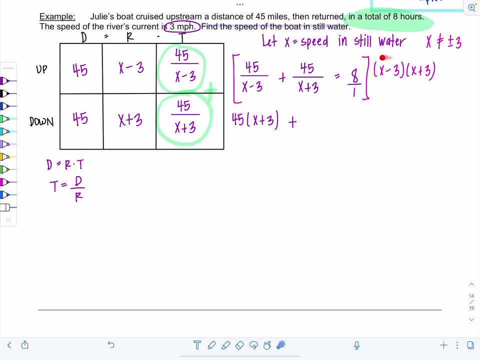 the x plus three will cancel. So I just have 45 times x minus three. Love it Equals eight times. nothing cancels You guys. okay, if we get this show on the road, I'm going to multiply out x minus three. x plus three, that's x squared minus nine. Okay. 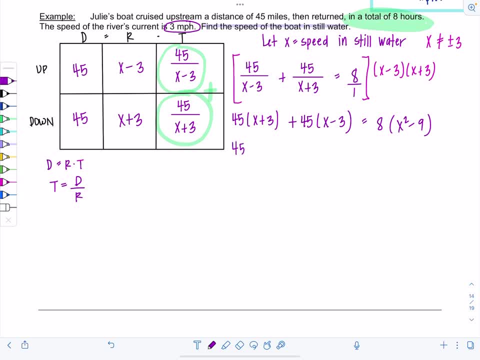 Good. So now let's distribute. We've got 45 x plus 45 times three. If you hit the gym, you're probably good at adding multiples of 45.. Okay so, 135 plus 45 times x minus three. 45 x minus 135 equals eight x squared minus 72.. 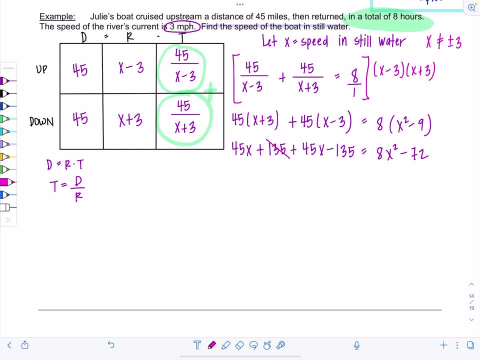 Nice. Okay, on the left hand side, notice the 135s. cancel out 45 x, 45 x, that's 90 x, And I see we've got an x squared. So we definitely are going to want to set this equation equal to zero. So let's go ahead and do that: Zero equals. 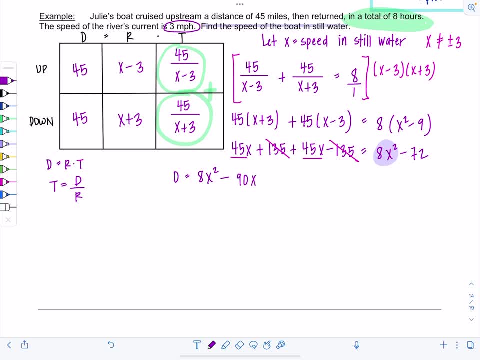 eight x squared minus 90 x minus 72.. Oh me, oh my, I'm not excited to factor this. Let's see: Can we divide out by some constant What's the biggest number that 890 and 72 have in common? It's just. 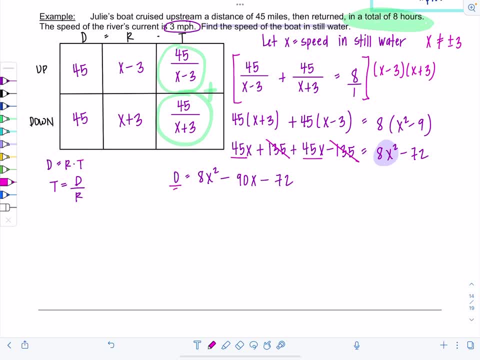 two. How depressing. Okay, So divide everything by two. It's the same as factoring out a two, but I like for it to just be gone right. Zero divided by any non-zero number is still zero, So zero equals four x. 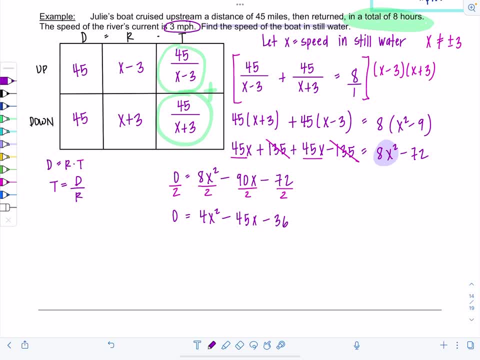 squared minus 45 x minus 36.. Okay, This can be a bit of a beast to factor. I don't want to do guess and check We could, but I'm going to review how to factor by splitting the middle term. Okay. 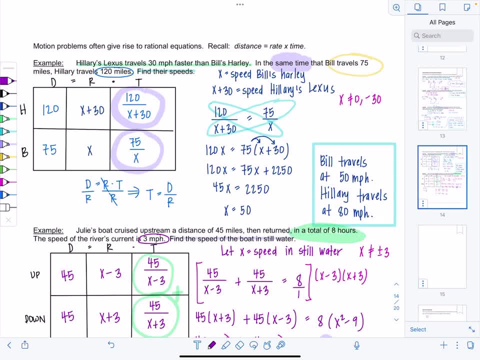 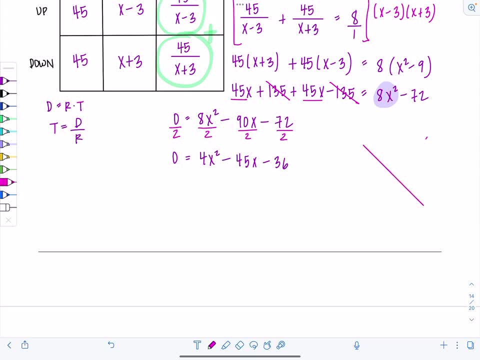 Let me add another little piece of paper here So we have room for this hot discussion. Okay, So as a review, when you factor by splitting the middle term, you here are the coefficients A. this is B and C, right For your trinomial. So A times C goes up here, Four times negative, 36,. 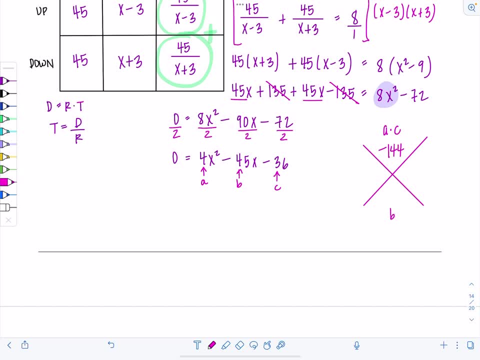 that's negative 144.. And B goes down here, negative 45.. B- Here's a bugs answer. B is equal to B equals 16.. You can do that if you want. F means return. we can say: But it's bearer function has to be bearer function as well. B means wasp, So we can do. 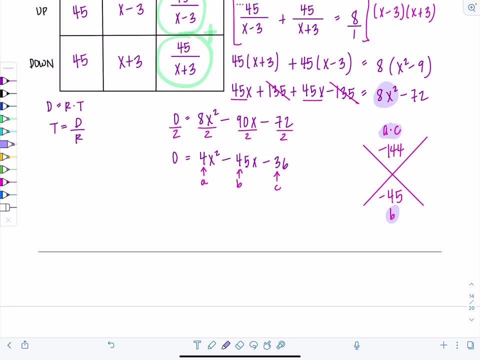 if so, B, 1, B- We can do if you can- and 144.. Is there any way that you can use those two numbers to add to negative 45? No way, no how. Next on the list: 2 times what is going to give you negative 144?? Well, 2 and 72.. 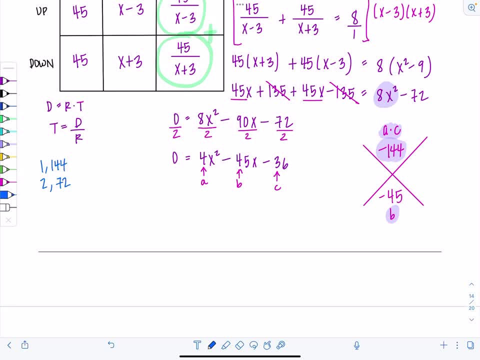 Is there any way I can add or subtract 2 and 72 to get negative 45?? No, Okay. next on the list: 3. Does 3 divide into 144?? If you don't know, check with your calculator or do some division. 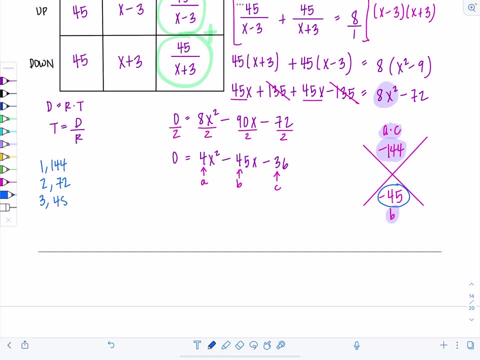 off to the side. 3 times 48 gives you 144.. Hmm, is there a way I could add or subtract those two numbers to get negative 45?? Why yes, I could use a negative 48 and a positive 3.. Perfect, 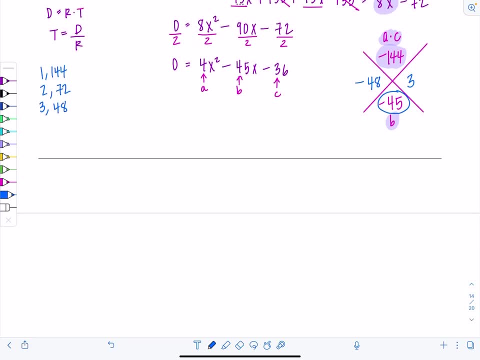 So what do we do with that now? Well, remember, we have this quadratic equation here. I'm going to split the middle term, I'm going to split the negative 45x using the two numbers negative 48 and 3.. This is what I mean. So we still have 0. 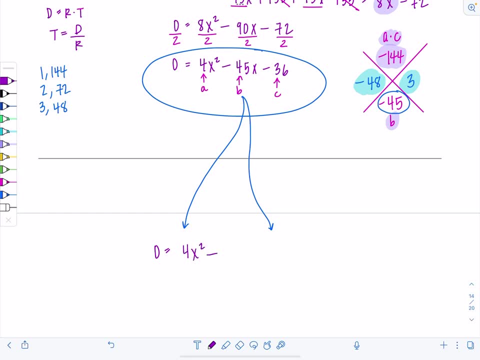 equals 4x squared minus 48x plus 3x minus 36.. So I used these two constants to split the negative 45x into negative 48x and 3x. This is still negative 45x, right? Yes, Why do I like this? 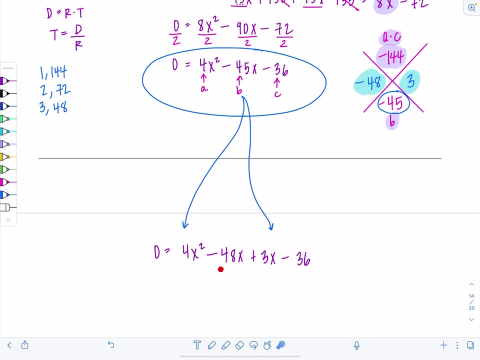 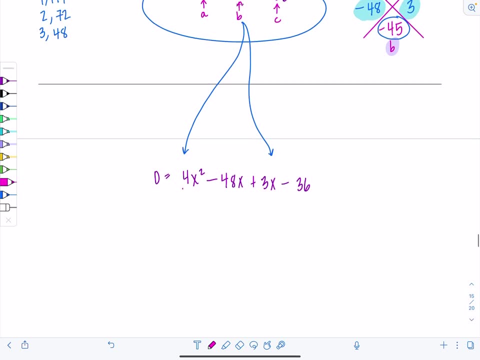 better, Because I have 1,, 2,, 3,, 4 terms I can factor by grouping. Grouping is where you take out the greatest common factor for the first two terms and then the greatest common factor for the second two terms. So let's see, What can I do? I'm going to take out the greatest common factor for the 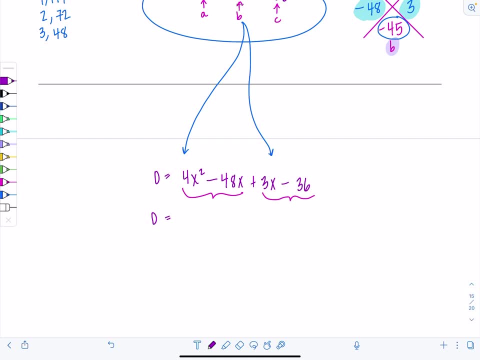 second two terms. I'm going to take out the greatest common factor for the second two terms. So I'm going to take out from 4x squared and 48x, What do they have in common? A 4x Good. So I'm going to take 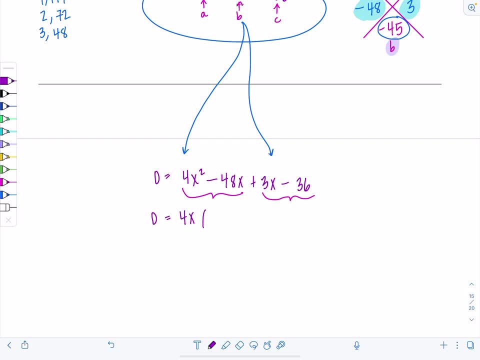 out 4x and I have left x minus 12, plus bring down that plus sign. what can I take out from 3x and 36? A 3,, right 3, and then you have x minus 12.. If you did all of the steps leading up to 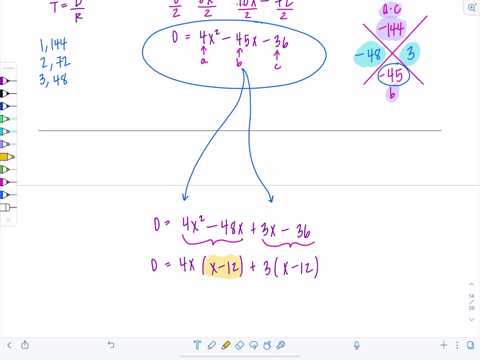 here correctly, then you should have the same result. So I'm going to take out 4x and I have the same factor up here, okay, This is why this factoring technique is so powerful, because sometimes guess and check can be a little tedious when you've got, you know, 4,. ooh, I didn't mean. 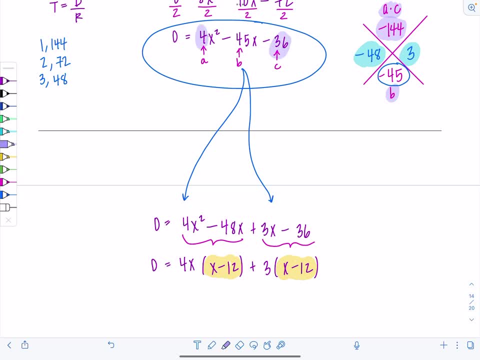 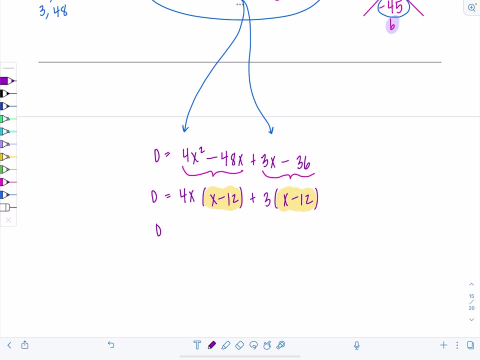 to x that out when you've got 4 and 36, which have so many possibilities. you don't want to sit there all day, you know guessing in vain. Okay, so now we're almost done, I'm going to take.